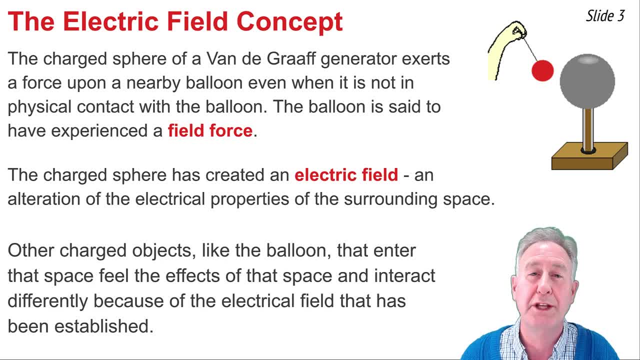 of the space that surrounds it, and any object, like the balloon, that's brought into that space feels the effect of the field and will interact differently because of the electric field. It's a way of explaining this somewhat awkward action at a distance that occurs despite any 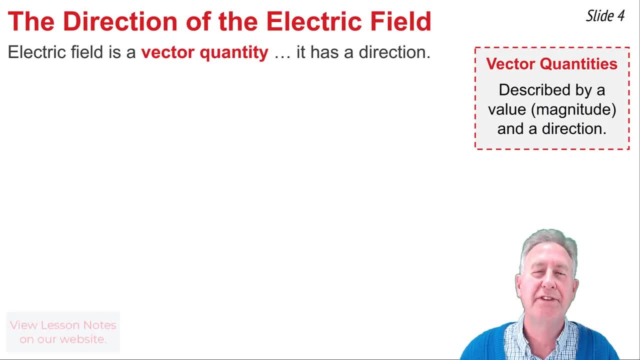 contact between the two objects. Electric field is a vector quantity. In describing it as a vector quantity, we mean that it has a magnitude or numerical value and a direction associated with it. The rule for the direction of the electric field at any given location in space around. 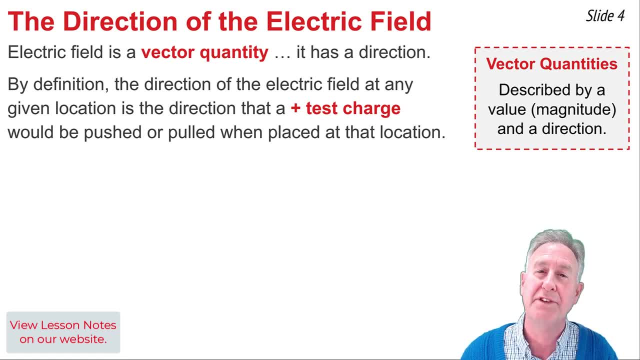 a source of charge is to say that it's the direction that a positive test object would be pushed or pulled when placed at that location. For sure it is. Here's a negative source of charge. Any positive test object would be pulled towards it. thus the electric field direction. 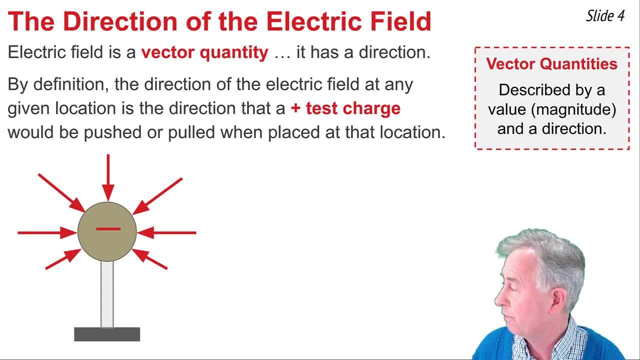 around this negative source charge is directed towards it. Here's a positive test charge. The direction of the electric field around it would be away from the positive force charge, since a positive test charge would be pushed away from it. In general we can say the direction of the electric field is always directed towards. 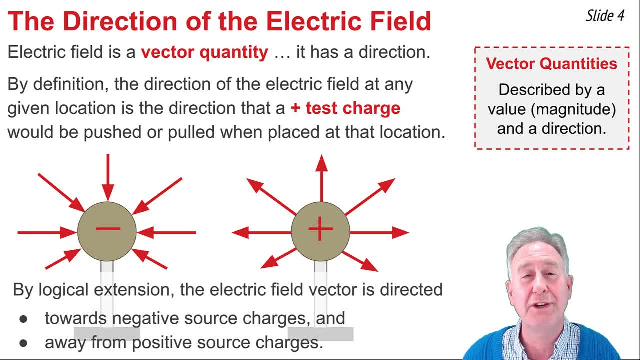 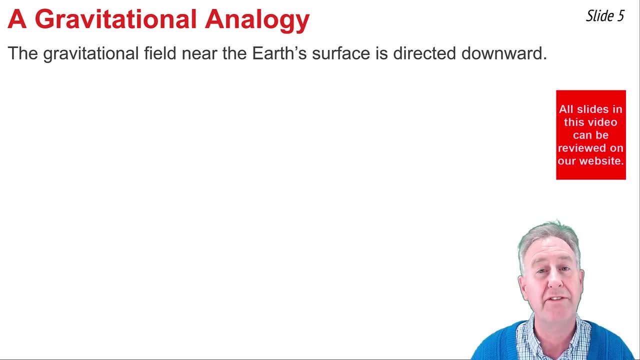 negative source charges or away from positive force charges. Well, we're done witharse Thanks. Bye for now. positive source charges. Gravitational fields are much like electric fields, but in the case of gravitational fields, the source of the field is a massive object and through its field it 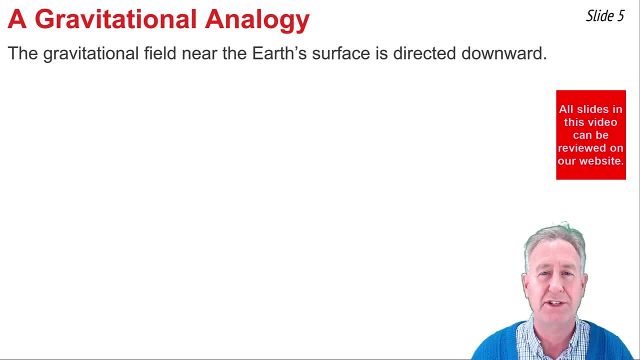 exerts action at a distance, forces on other masses Around the surface of the earth, the direction of the gravitational field vector is directed downwards. So if we were to consider a case in which an object moves from a high elevation to a low elevation, this would be a movement in the 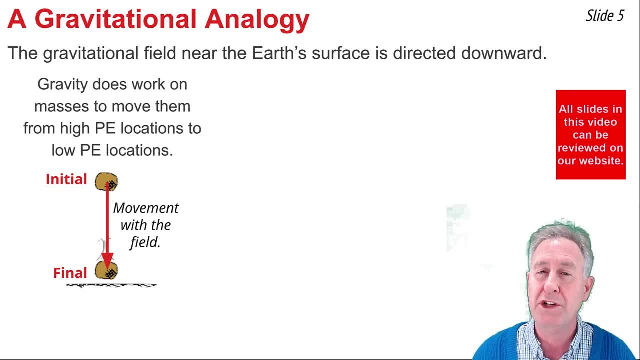 direction of the gravitational field. Such a movement occurs naturally and does not require the exertion of an external force. Gravity, acting through its field, does work on the object to move the object from a high potential energy location to a low potential energy location. If we consider: 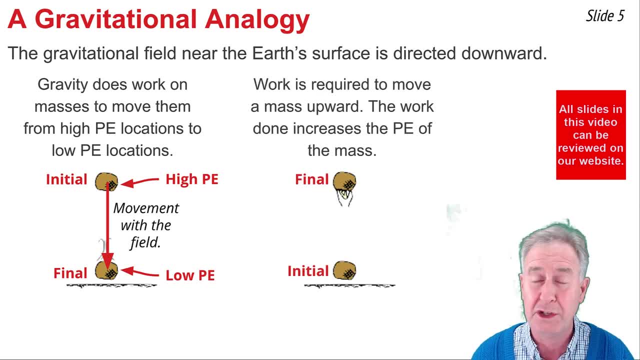 the opposite case of an object moving from a low elevation to a high elevation. this would be a movement against the gravitational field. In such a case, an external force would have to do work to move the object from a low elevation to a high elevation. 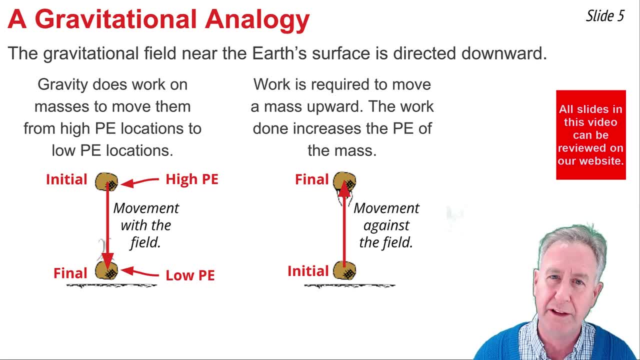 In such cases, the work adds potential energy to the object, moving it from the low potential energy location to a high potential energy location. One of my main points in using this gravitational analogy is to emphasize that the movement of a mass within a gravitational field is always. 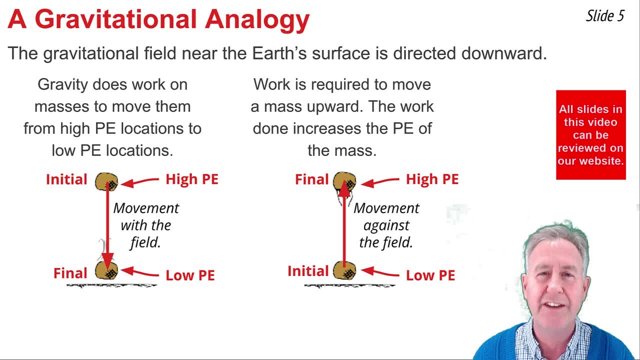 accompanied by a change in potential energy. If the mass is moving from a low elevation to a high potential energy location, the mass moves in the direction of the gravitational field. This is a loss of potential energy. If the mass moves uphill, against the direction of the 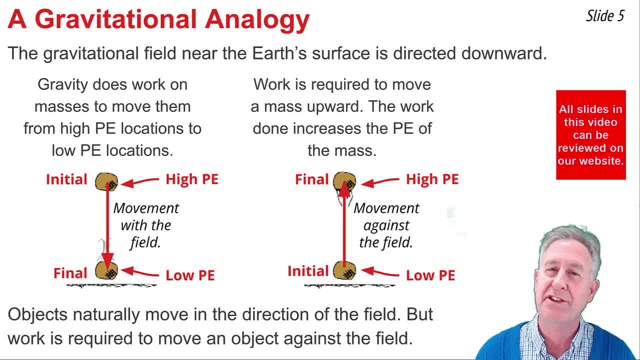 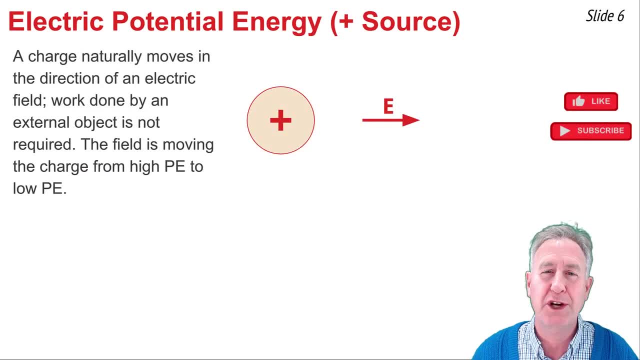 gravitational field, there is a gain in potential energy, as that external force does work upon the mass. In an analogous manner, whenever an electric charge moves within an electric field, there is a corresponding change in electrical potential energy. For instance, if we had a charge at location A and 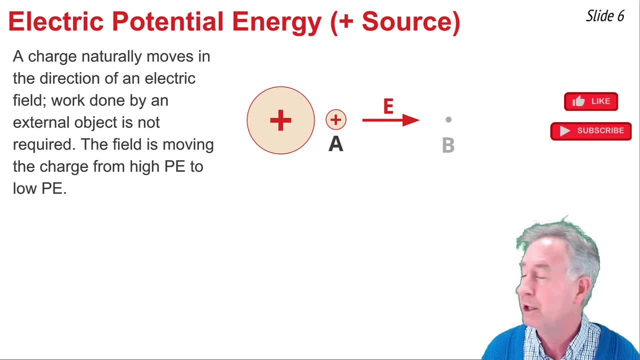 moving with or in the direction of the electric field to location B. that would not require work by an external force. That would happen naturally, since the motion is in the direction of the electric field. That would be analogous to moving downhill. That would be a motion from a high potential energy location to a low potential energy location. 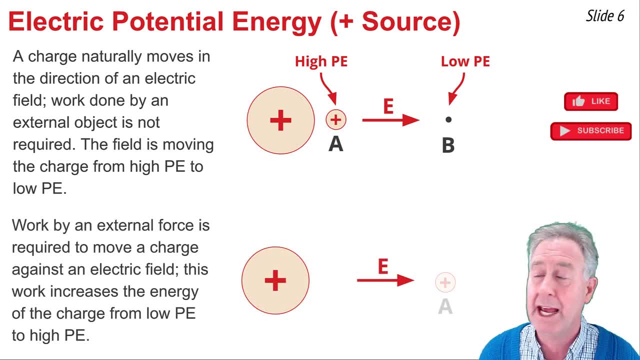 In contrast, if we had an electric field and there was a mass at location A and moving against the direction of the electric field, that would require the exertion of a force by some external source and work would be done by that force to add energy to the object. 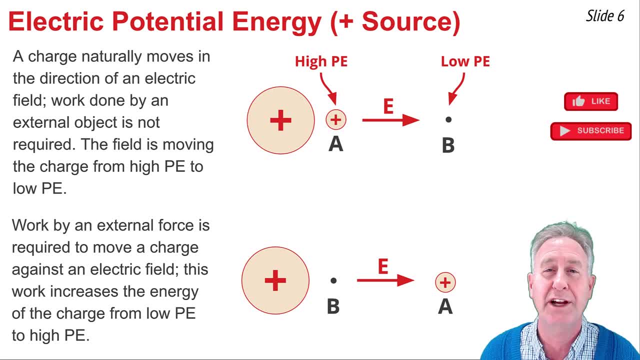 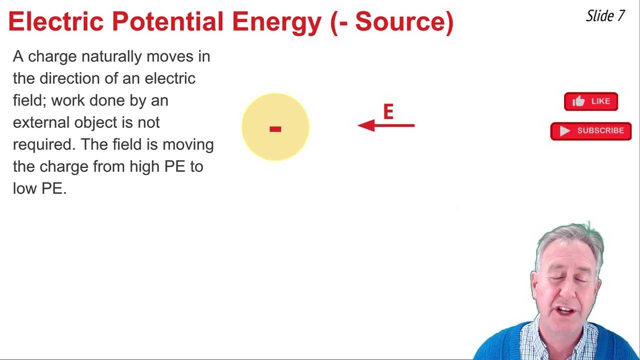 In such a case of the charge moving against the electric field, the charge would be moving from a location of low potential energy to a location of high potential energy. We just saw situations in which the electric field was created by a positive source charge. Now we'll consider situations where we have positive test charges moving within a field that is created by a negative source charge. 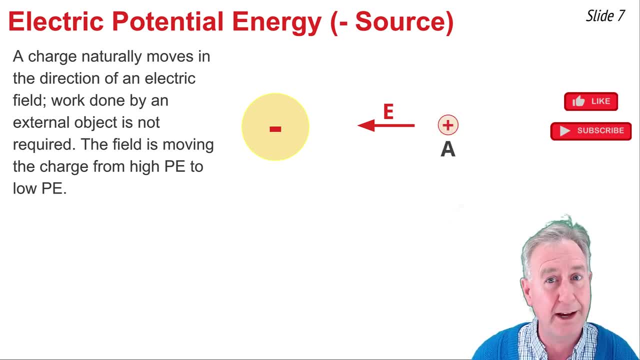 In the first case we'll consider an object starting at A- a positive test charge- and moving with the field towards the negative source charge to location B. In this situation the movement is with the electric field. It's analogous to a mass moving downhill. 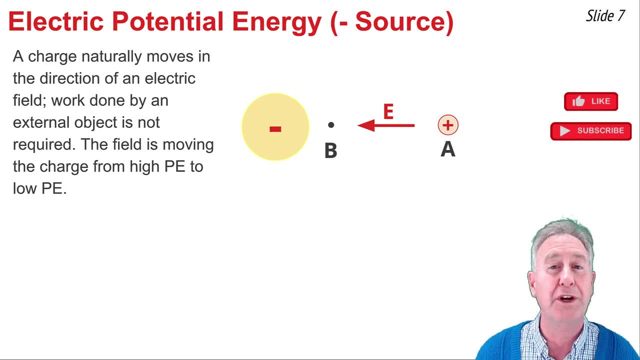 It would not require work done by an external force, but would occur naturally with the help of the electric field. It would not require work done by an external force, but would occur naturally with the help of the electric field. It would not require work done by an external force, but would occur naturally with the help of the electric field.